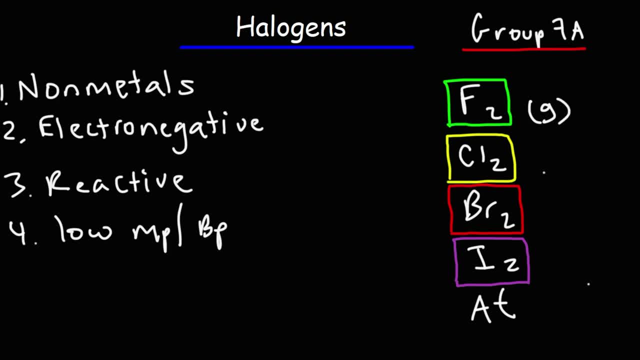 So remember the physical states of these gases. Fluorine is a gas, Chlorine is a gas, Bromine is a liquid. Iodine is a solid. Acetine is a radioactive solid. Now, as you go down the group, the boiling point increases. 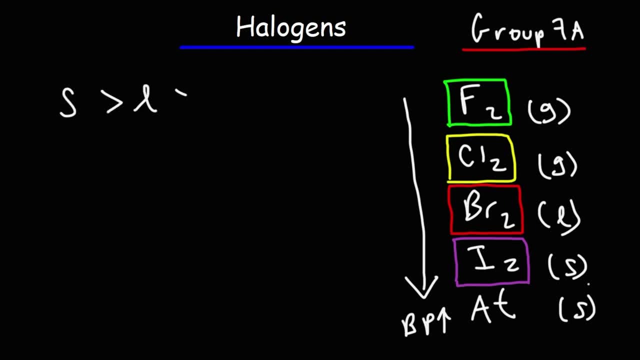 Solids have higher boiling points than liquids, and liquids have higher boiling points. The fact that fluorine is a gas at room temperature tells you that it has a low boiling point, Iodine being a solid that tells you that it has a higher boiling point than fluorine. 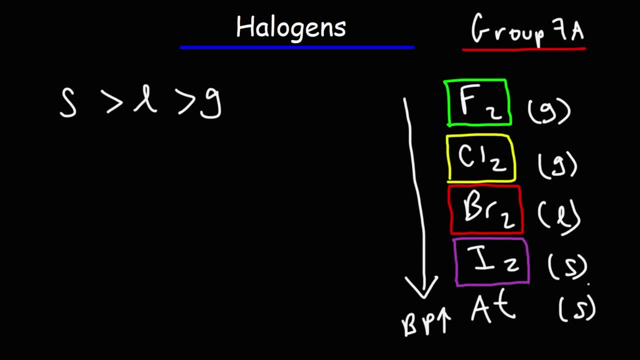 So the boiling point of the halogens increases as you go down. As you go down the group, the atomic radius increases. So iodine has a higher boiling point than fluorine. It's also bigger in size relative to fluorine. As you go up the column, electronegativity increases. 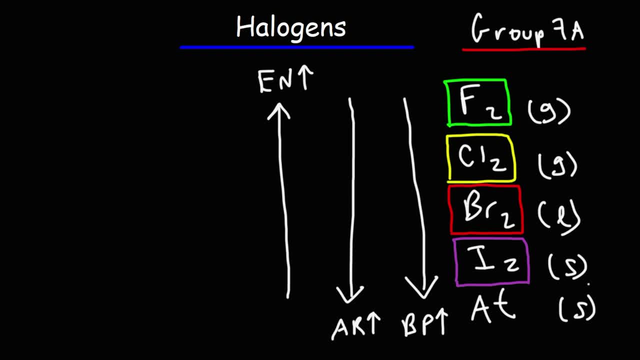 Fluorine is more electronegative than chlorine, Chlorine is more electronegative than bromine, and so forth. In fact, fluorine is the most electronegative element on a periodic table. According to the Pauling scale, it has a value of 4.0. 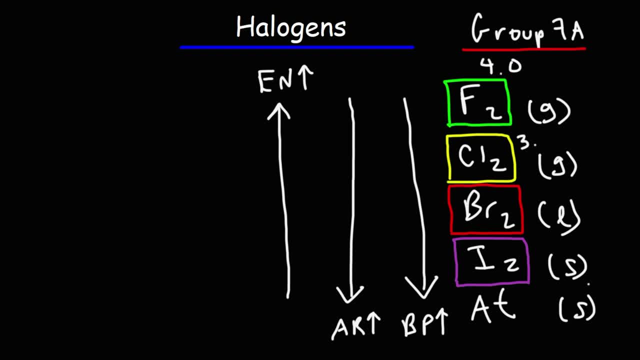 For chlorine, its electronegativity value is 3.0.. Bromine is 3.0.. Bromine is 2.8.. And for iodine it's 2.5.. So those are the electronegativity values of the common halogens. 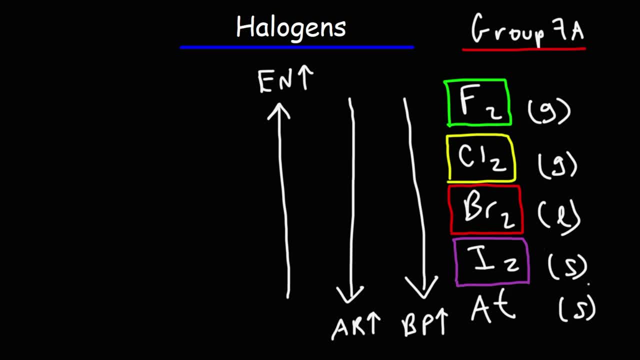 Acetine is radioactive, so it's typically not used very often. Now the next thing we need to talk about is the reactivity. The reactivity of the halogens increases as you go up, So fluorine is more reactive than chlorine. Chlorine is more reactive than bromine. 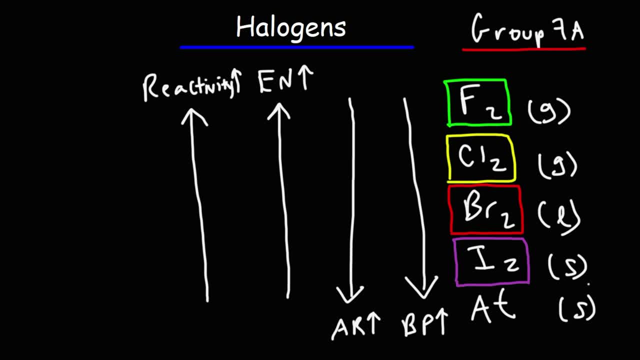 Now it's important to know this when, especially when, you're dealing with the displacement reactions of the halogens. Now let's talk about that. So remember, reactivity increases as you go up. I'll put an R to represent reactivity. So, because chlorine is more reactive than bromine, 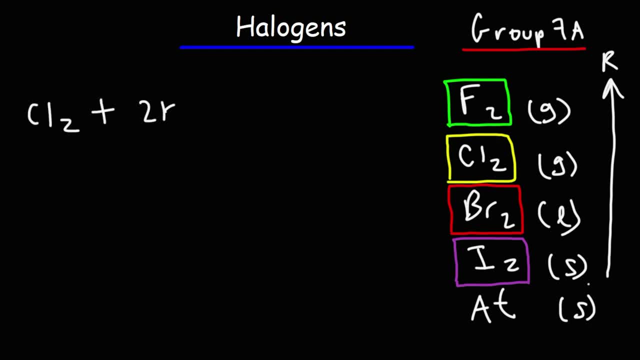 Chlorine is more reactive than bromine. It can displace bromine in a single displacement reaction. So let's say you have an aqueous solution of potassium bromide and you pass chlorine gas through it. Chlorine is going to displace the bromide ion out of the solution. 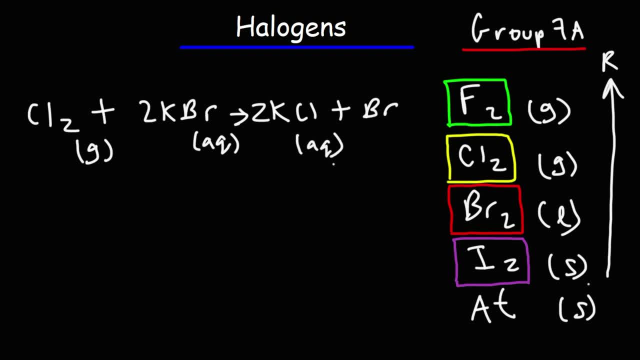 So you're going to get potassium chloride instead of potassium bromide, and bromine is going to form as a red liquid. So the chlorine gas kicked out the bromide ion out of the aqueous solution, pushing it into its elemental form. Now let's say if you were to take iodine. 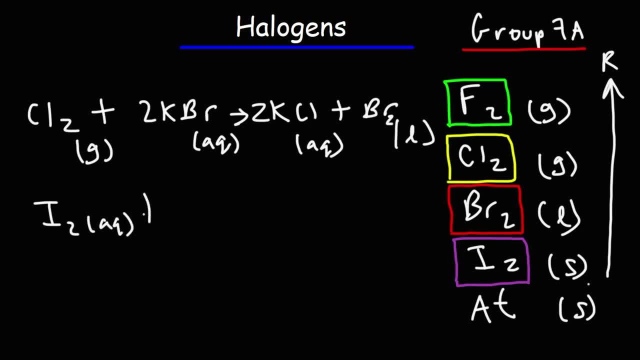 Let's say in its aqueous form. let's say it's dissolved in water. You can dissolve it in the form of the triiodide ion. But let's say you put it with potassium bromide, Will it form potassium iodide? 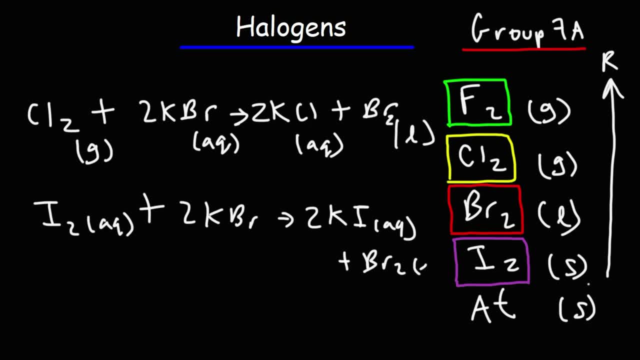 Will it displace bromine out of the solution? What would you say? The answer is no. This reaction will not proceed. as written. Something that's less reactive cannot form something that's more reactive Without the input. This is not a spontaneous reaction. 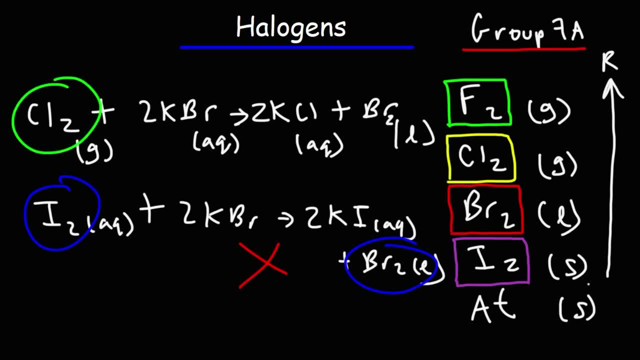 However, something that's more reactive can create something that's less reactive, So this reaction will proceed as written, but the other one won't. So because iodine is less reactive than bromine. iodine cannot displace bromine out of the solution. 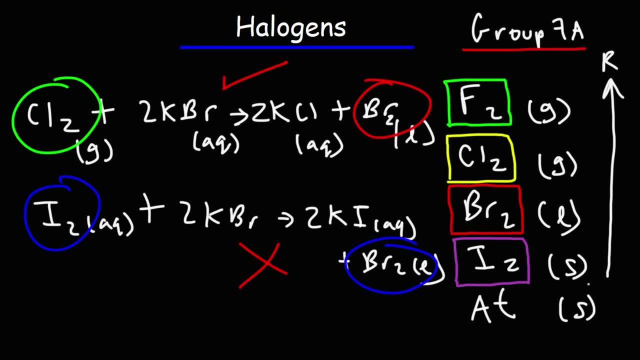 Chlorine is more reactive than bromine, So chlorine can displace bromine out of the solution. The reason is because if sodium is more active than sodium bromide, Chlorine is more active than potassium boron. Now the halogens can be acting with hydrogen as well. 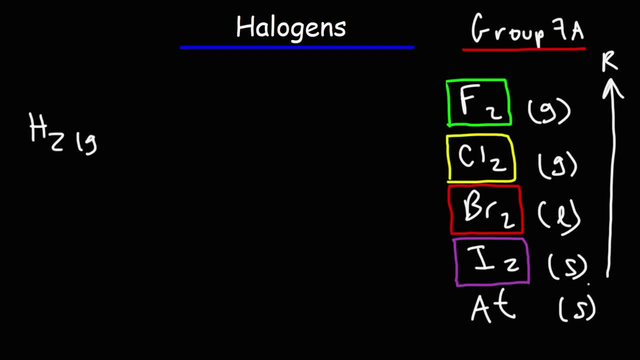 So this is this: When hydrogen gas reacts with bromine, An acid will form. We're going to get hydrobromic acid. Now, this is normally a gas. न you dissolve it in water, it will be aqueous. Hydrogen can also react with chlorine to form. 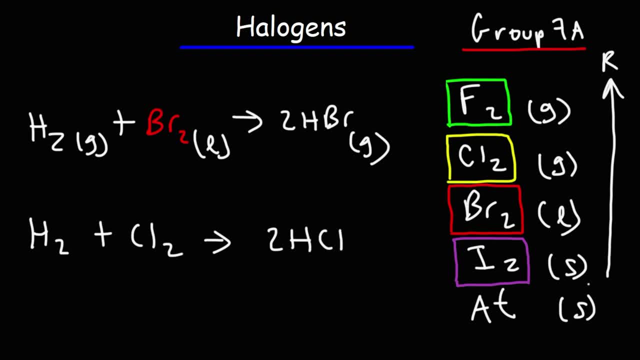 an acid, hydrochloric acid, which is also a gas and can also dissolve in water. Now the halogens can also react with metals. When sodium metal reacts with chlorine gas, sodium chloride will form. Sodium chloride is table salt. So any time a halogen reacts with a metal it'll create some. 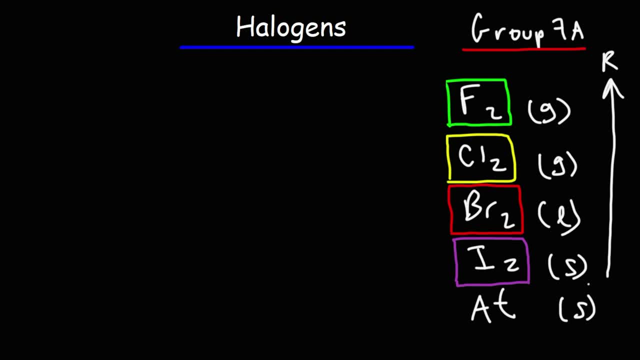 type of salt. Now the halogens. they have seven valence electrons and they only need one more electron to satisfy their octet requirements. So they need one more electron to have a complete outer energy level, And so they tend to be very reactive. They really want that electron and thus their electronegative 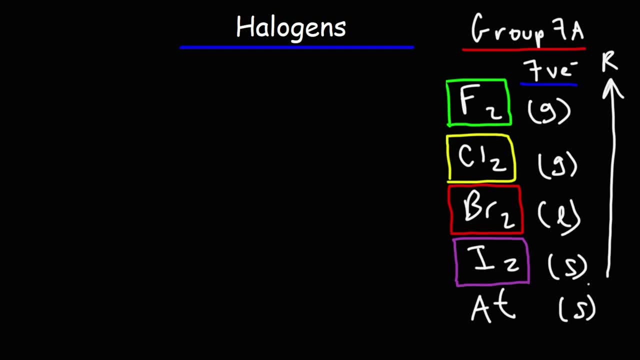 Electronegativity is the ability of an atom to attract an electron to itself. Non-metals, typically, are electronegative. Non-metals like to acquire electrons, whereas metals like to give away electrons. When a fluorine atom acquires. 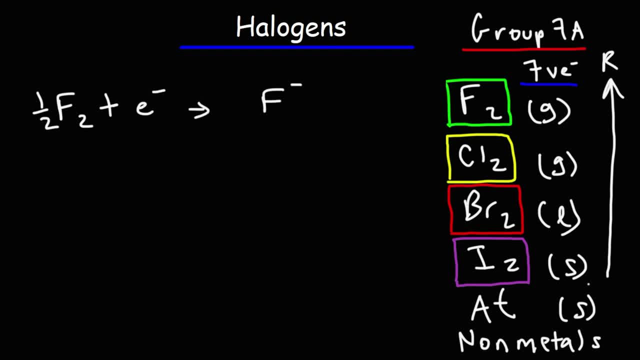 an electron, it becomes fluoride. Same is true for chlorine: When it takes an electron, it becomes chloride. When it takes an electron, it becomes chloride fluoride. So because they only want one electron, they typically form anions with a negative one charge, but their oxidation states is not limited to negative one In the case of 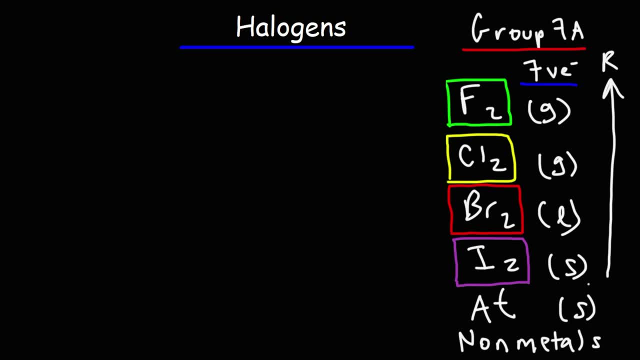 fluorine, yes, but for the heavier elements, like chlorine, bromine, iodine, they have access to the D orbitals so they can have multiple oxidation states. As a pure element, the oxidation state is zero. As an ion, it's minus one after they acquire one electron.